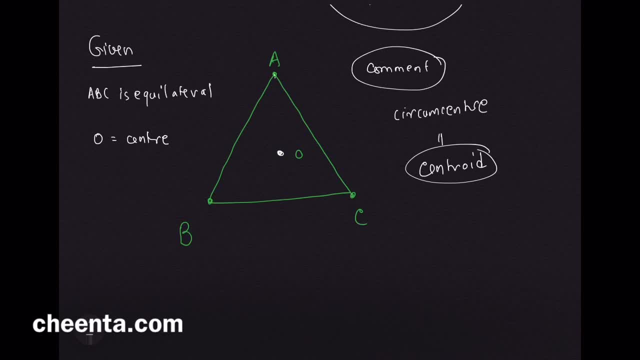 thing, since the triangle is equilateral, and what we want to do is we want to fold A, B and C in such a manner that A falls on O, B falls on O and C falls on O, and so on. so now you can see that the circumcenter has a big triangle on it, and 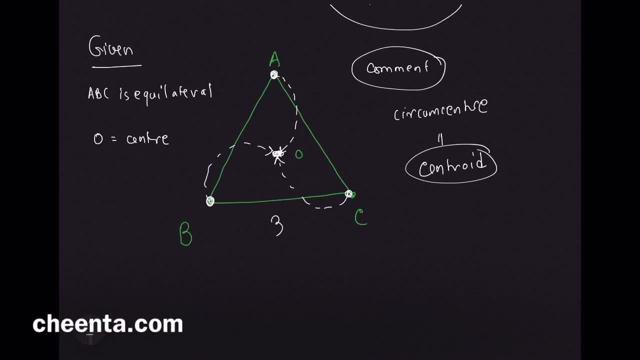 you can now see that the right side of the right side of the right side has the circumcenter, and the next thing that we want to do is to get a picture of the resultant picture is. whatever the resultant picture is, we want to find out the area of that. oh, it's also given that the perimeter of 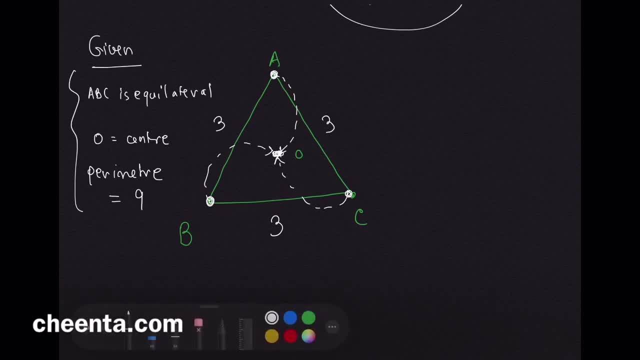 video and you're strongly suggested to try it first. so the goal: find the area after the folding. and how is it folded? as i mentioned, a goes to o, b goes to o and c goes to o. it's actually not a very hard problem now, assuming that you have tried this. 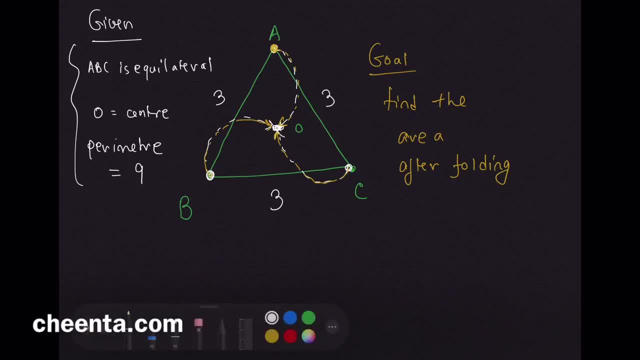 problem on your own. i'll go ahead and give you a clue so that you can actually try it one more time. the clue is when you are folding. this usually means find the midpoint. i mean, it's a very crude way of saying it, and i'll tell you exactly what it means in this context. 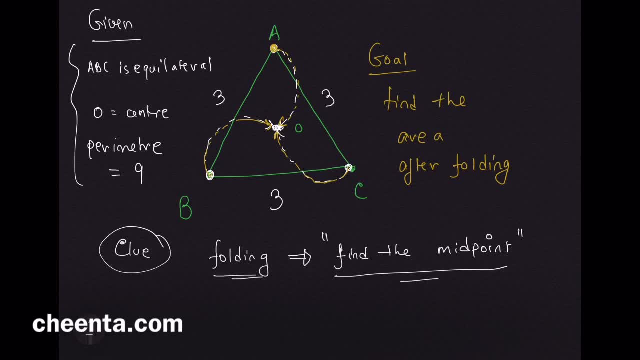 but usually folding means it's, it's getting reflected in some sense reflected. so what does it mean in this picture? well, let's join bo, let's join bo. uh, in fact, if we produce bo, let's delete this little m arrow part. if we, if we produce, 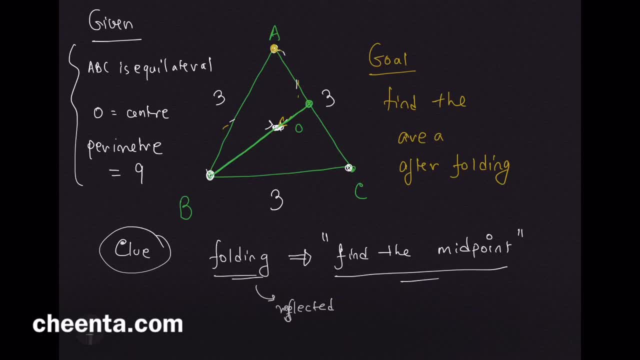 b? o it hits the midpoint of ac. let's call that point d. all right now we know that the triangle is, uh, three, three, three equilateral. so this little part is three by two and you can easily check that this triangle will not be an equal triangle. 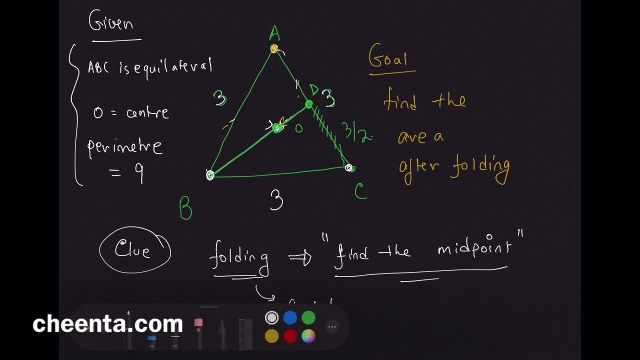 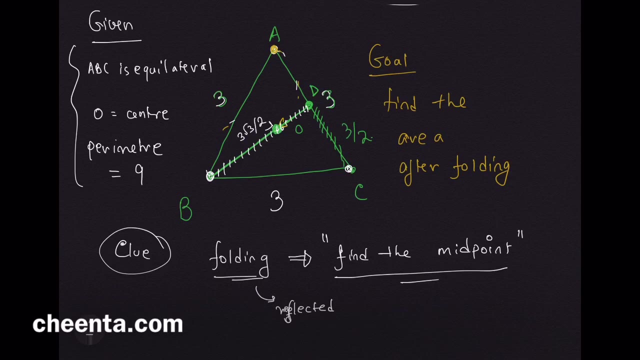 co this part, the perpendicular, and that's because the triangle is equilateral. This perpendicular is 3 square root of 3 over 2, the length of the perpendicular, and it's a very easy application of Pythagoras theorem on this triangle. So apply Pythagoras theorem on triangle BDC. 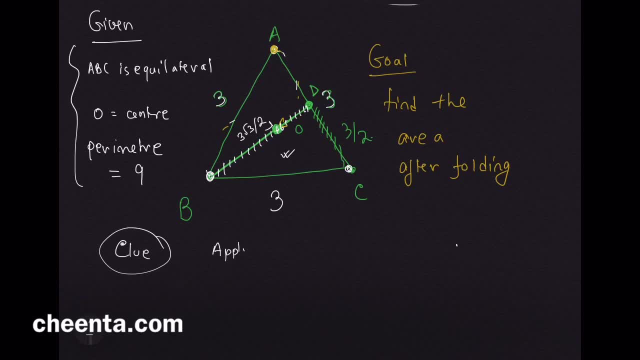 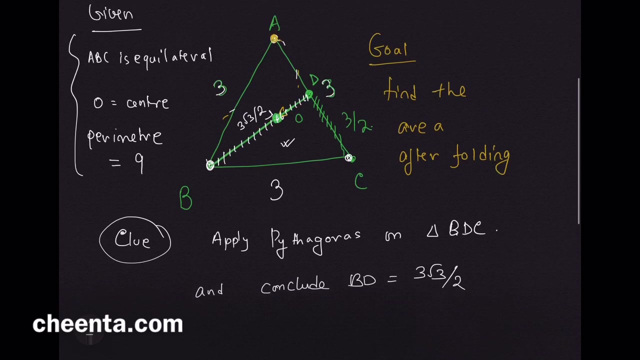 maybe you can write that: apply Pythagoras on triangle BDC and conclude that BD is 3 square root of 3 over 2.. All right, all that's good. Now we are trying to fold this B so that it falls on O. How? 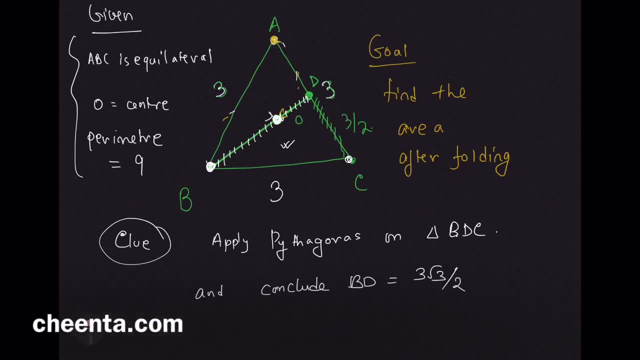 do you do that? Okay? so what essentially you have to do is find the midpoint. maybe I can just draw this, the midpoint M of BO and that's, and draw a perpendicular to the point M. Now you see what I am saying, right? I mean BM folds to MO and that makes B exactly. 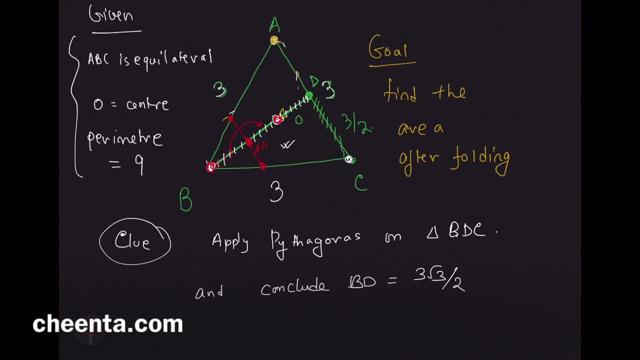 fall on O. Why? Because this is the. this M breaks BO into exactly two equal parts, So a little bit of imagination will be necessary. So you are in your final picture and you can see that after you have folded, maybe I can just use a little bit of color- this part will be. 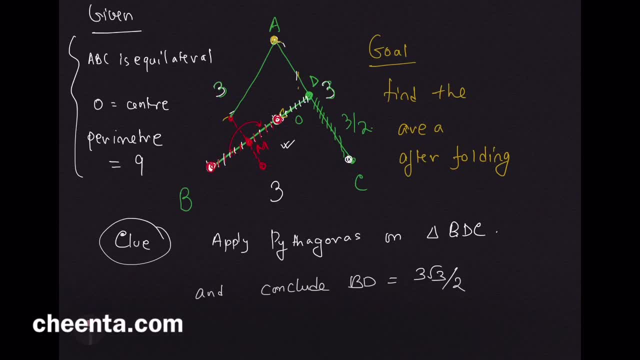 there and again, this part will be there, but this little part right here will be vanished, right, Because you have folded it and it sort of will fall on O, and this little part will be vanished, and similarly here, everything here will be vanished, Similarly here, everything in this. 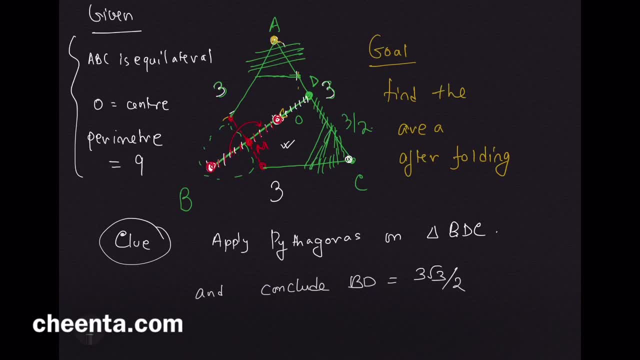 portion will be vanished, and you will be, you will get a hexagon in some sense, and what we will do is we will find the area of this vanished portion and then, by symmetry, all of this portion will be told here that the area of this feature that we were talking about is equal. We'll say all of this. 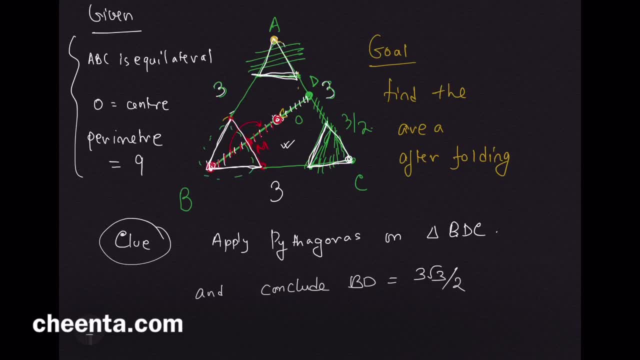 vanished pieces. all of these vanished pieces will be of equal area and then obviously delete these vanished pieces from the main area. that's idea. So if each vanished piece is of area Delta, then from the area of triangle ABC delete three Delta right. So, delta, you cancelled. So you finish dealing now with these pieces. and what you did, is you what? you become a group of the factors here, right? So you haveoll הזה. we have done something. also, please don't forget that if you have done something else, then please complete Compact steps. 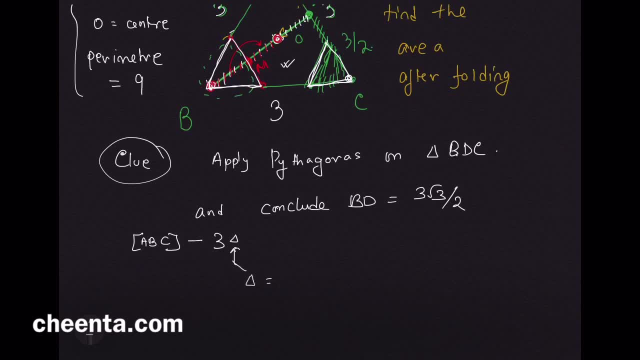 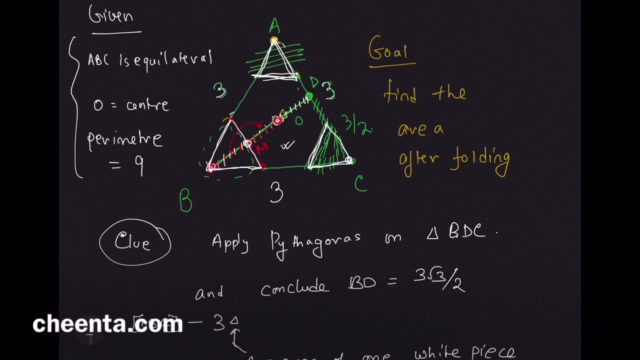 So delta is this? delta is the area of one white piece. right, Okay, now you can just pause the video here and give it a try. It's not very hard anymore. Okay, so this point is the midpoint of BO. 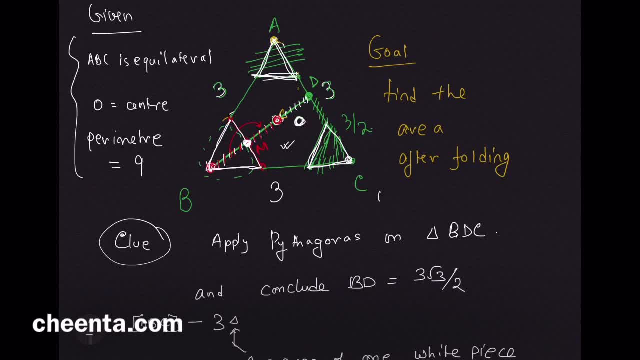 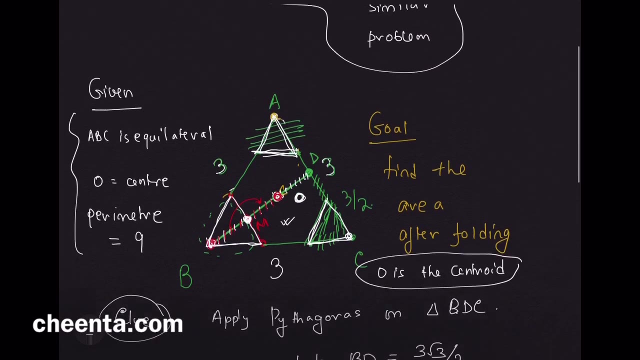 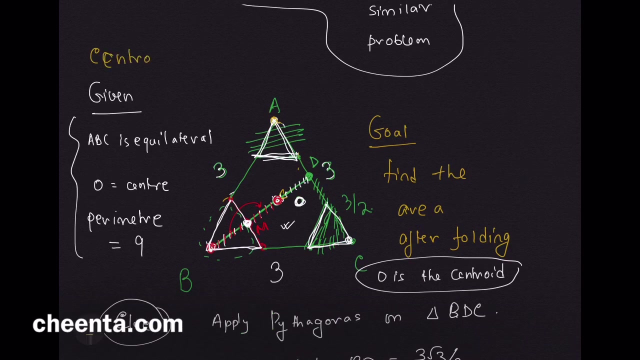 And remember O is also the centroid, is the centroid Because, as the triangle is equilateral, the centroid, the orthocenter and the circumcenter all are coinciding. Okay now we will use now a result from geometry that centroid divides median median in 2 is to 1 ratio. 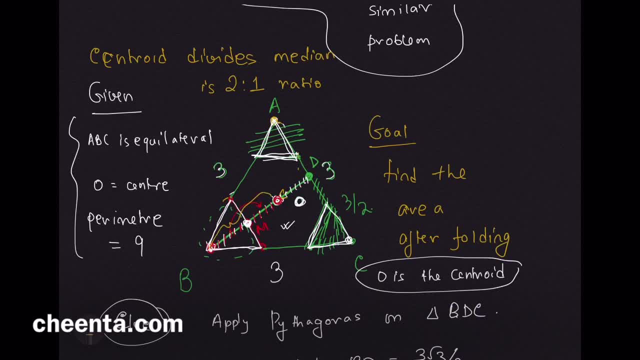 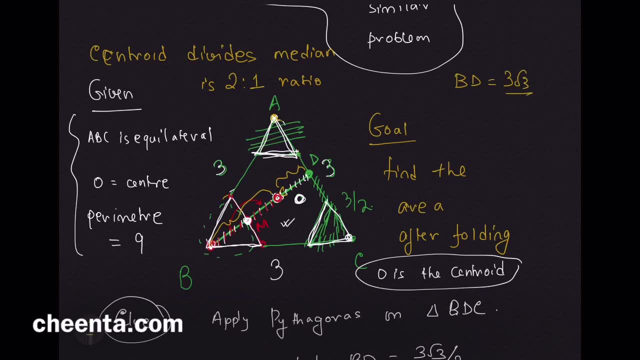 Okay, So this BO is 2 parts and this OD is 1 part. We know that BD is 3 root 3 by 2. We computed that And then this BD BO is 2 third of that. But M is the midpoint of BO, right. 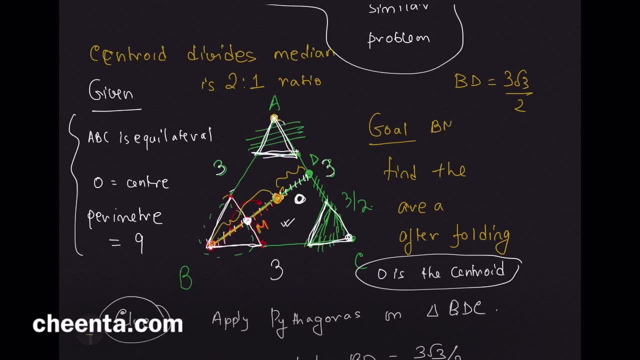 M is the midpoint of the BO, So BM is exactly 1 third of BD. This is 1 third. This was 2 third. You break it into 2 parts. Each is 1 third, right, Okay? So BM? so BM is exactly square root of 3 by 2.. 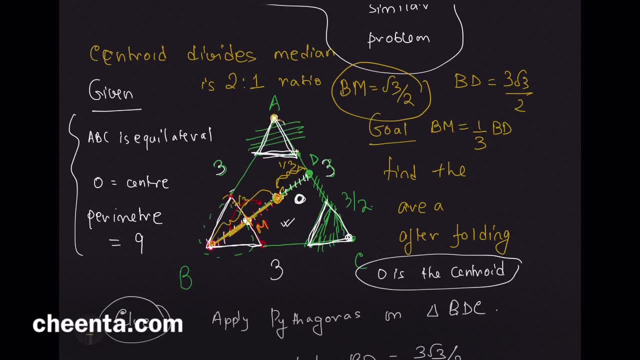 Excellent. Now you can go to the link in the description to finish off this problem on your own. We put more hints there, But we don't want you to give the entire solution, because that's kind of that will. that will ruin the entire story. 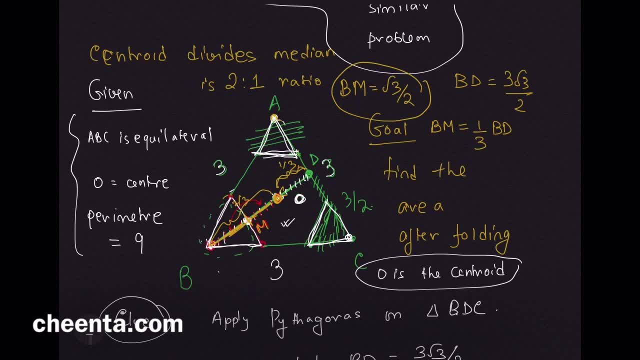 Okay, Maybe one more hint. The other hint is this triangle that we, this white triangle, is similar to this big BAC triangle And we already know that this perpendicular is 1 third of this perpendicular. So, clearly, by similarity of triangles, 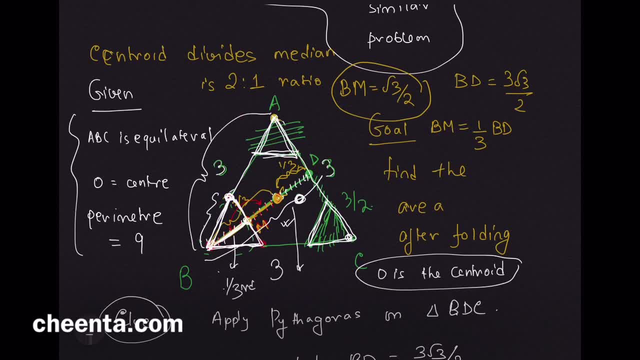 this little portion is 1 third of this one, So it's exactly 1.. Okay, So now you should be able to finish this off, because this is an equilateral triangle. by similarity, It's white, 1.. Each side length is 1.. 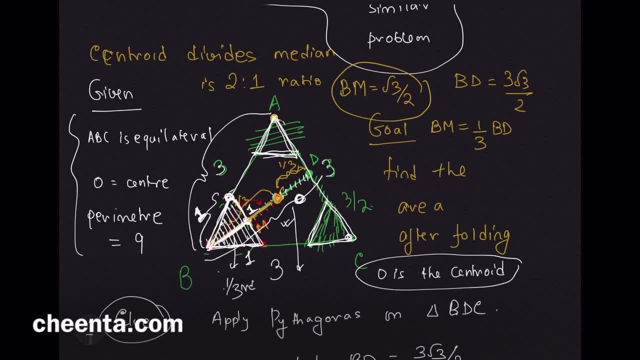 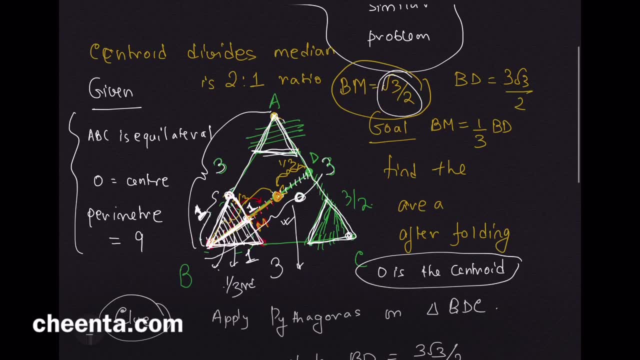 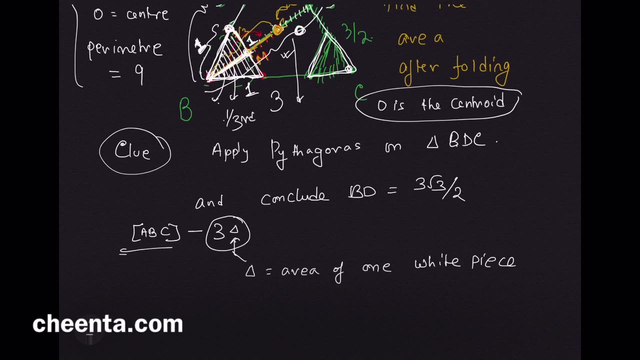 And, and the height is square root of 3 by 2.. We know that This is the height, So you know the area of this white piece. Now multiply that by 3 and delete it from the triangle ABC's area. 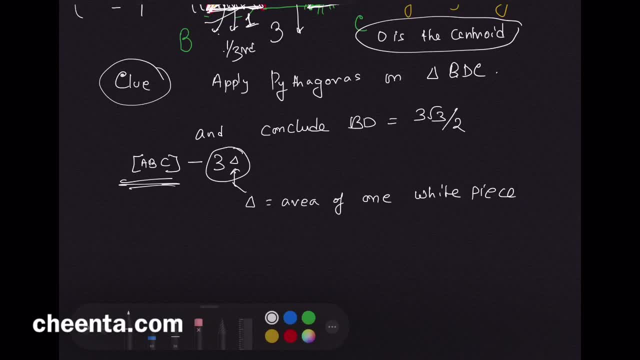 I'll give you the final answer so that you can test it on your own. So the final answer is 3 square root of 2, square root of 3 over 2.. This is the area of the folded piece paper.